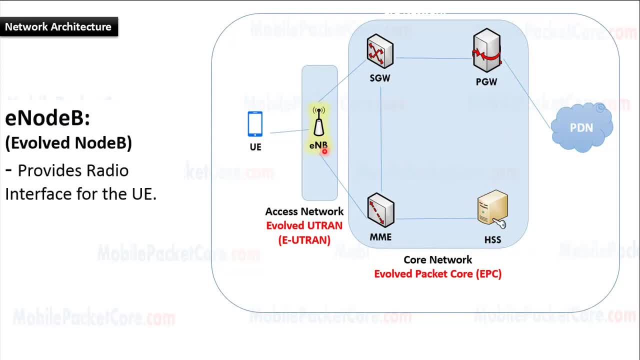 HSS. First, the UE connects to the E-NodeB. The E-NodeB provides the radio interface for the UE and the E-NodeB connects to the MME. MME refers to mobility management entity. The MME is the entry point. 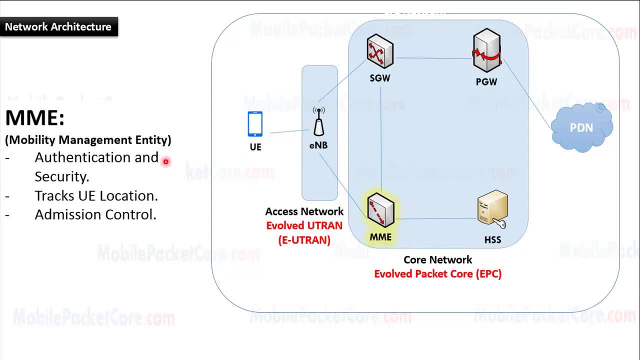 for the evolved packet core. It performs authentication and security. The MME authenticates the UE and performs security procedures in order to secure the messages sent and received to and from the UE. In addition, the MME connects to the E-NodeB. The E-NodeB is the entry point for the 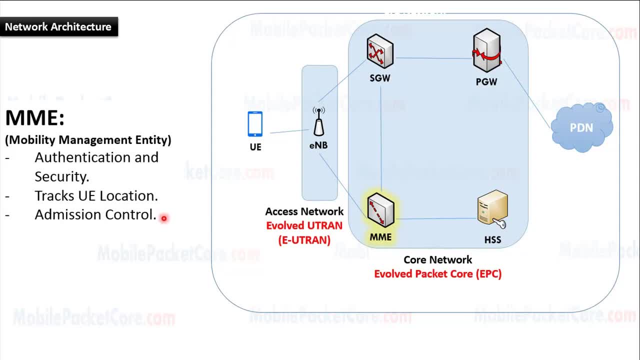 MME. The MME tracks the location of the UE and performs admission control, which means it decides if the UE is authorized to access this network or not and if network resources should be allocated to this UE. The MME connects to the HSS and the SGW. The HSS refers to home subscriber server. 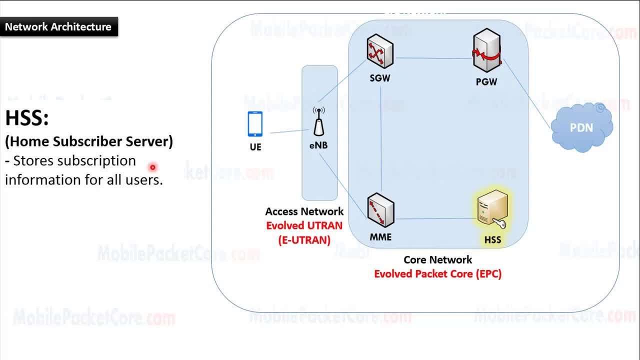 It contains a database that stores the subscription information for every user in the network, while the SGW refers to serving gateway. During session establishment, the MME will exchange signaling messages with the E-NodeB and the SGW and will instruct the E-NodeB and the SGW to establish a tunnel to directly pass user plane. 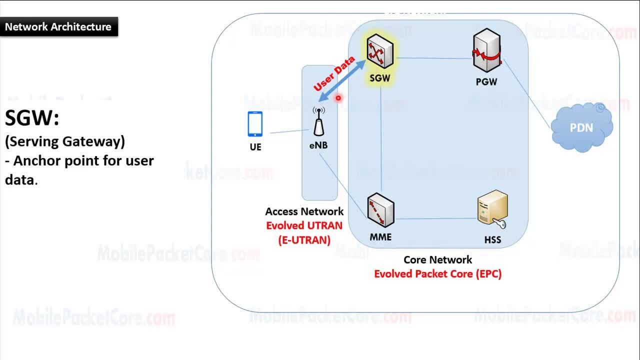 data between each other, so that user data will move directly between the E-NodeB and the SGW without passing by the MME. Therefore, the SGW is the first point in the evolved packet core that receives user plane data from the E-NodeB In turn. 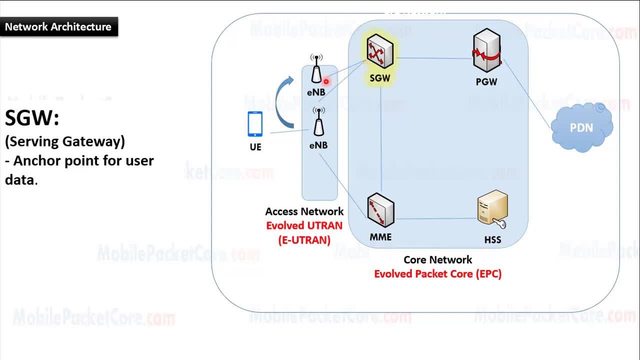 the SGW serves as the mobility anchor point for user data while the UE is moving between different E-NodeBs. Then the SGW connects to the PGW, which refers to PDN gateway. The PGW connects between the core network and the PDN. Finally, the PDN refers to public data network. It is the external network. 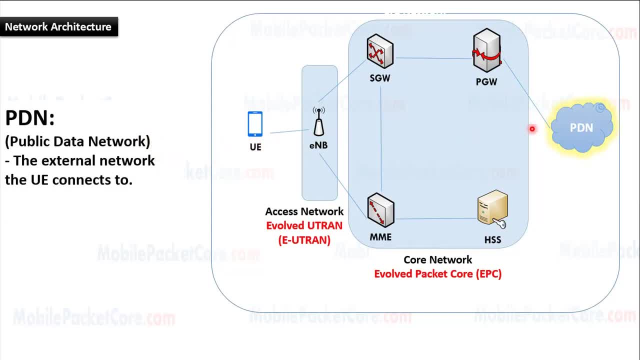 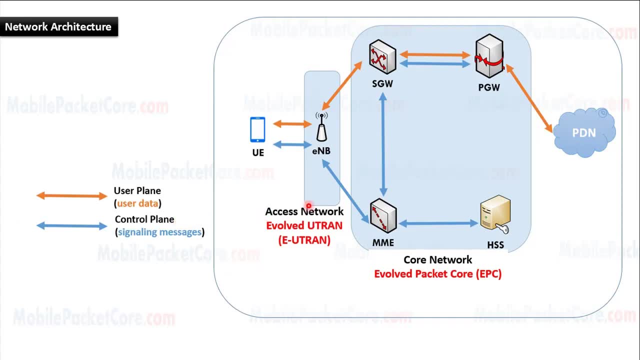 the UE connects to, if it is the internet or any other network. In summary, the nodes will use the control plane to pass signaling messages between each other, And the path of the signaling messages will be from the UE to the eNodeB, which provides the radio interface for the UE, Then from the eNodeB.